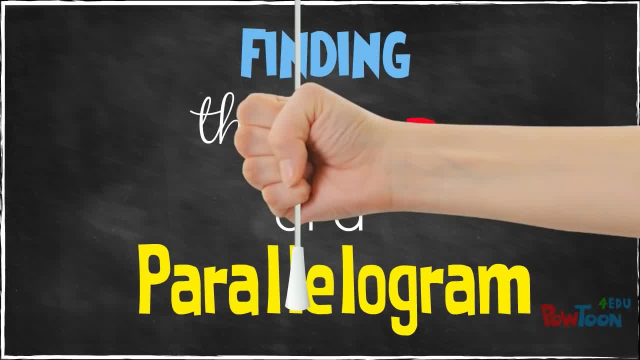 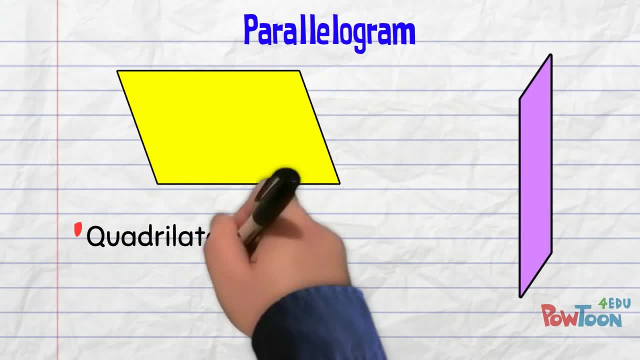 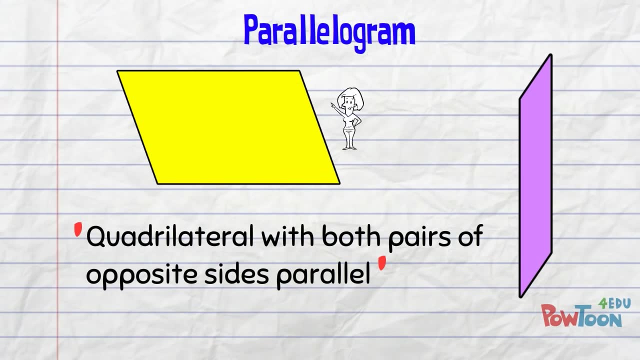 Finding the area of a parallelogram. This is a parallelogram, So is this A parallelogram? is? It looks a bit like a rectangle that's been nudged over. How can we find the area of a parallelogram? 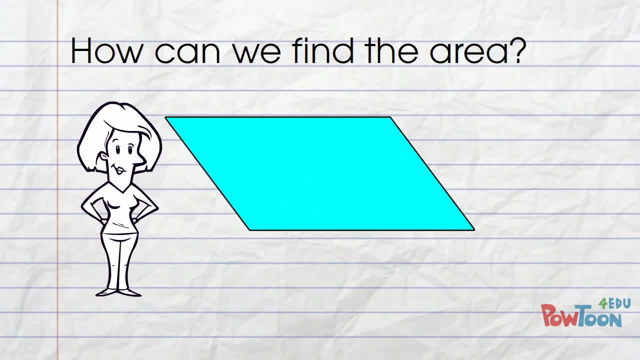 Well, don't be put off by the sloping sides, Because here's a way of thinking that's going to help you. If I cut a triangle off this side and move it over to this side, we get a form that is so much easier to work with. 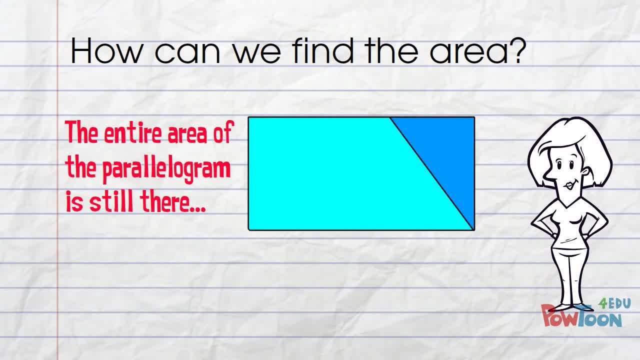 I didn't take anything away. The entire area of the shape is still there. I just rearranged it to form a rectangle, And you know how to find the area of a rectangle Length times width. But for a parallelogram we say the area is: 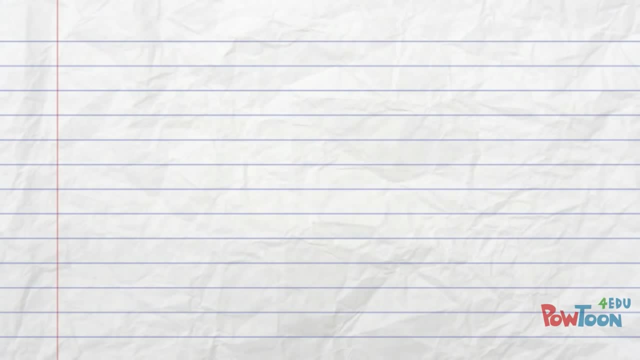 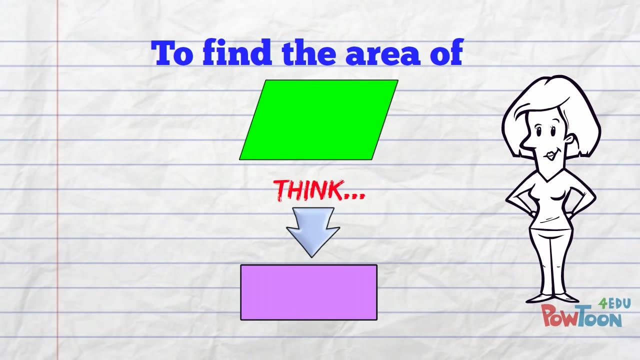 Base times height. When we have to find the area of a parallelogram, we think of it like a rectangle. Like I just showed you, A rectangle has right angled corners, So we have to form a right angle. We find the base. 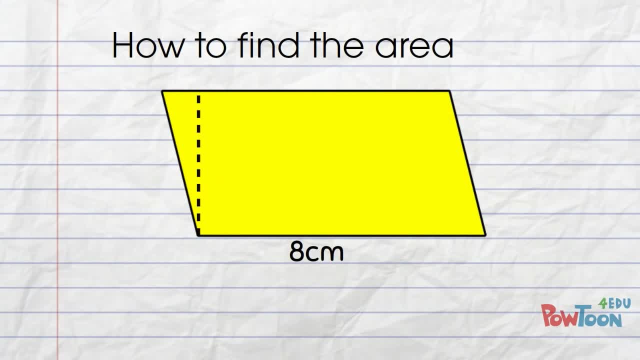 Here it's 8cm. And then we run a perpendicular line off the base to get the height. The height forms a right angle with the base, Just like the right angled corners of a rectangle. That is a key point to remember. So here's our height. 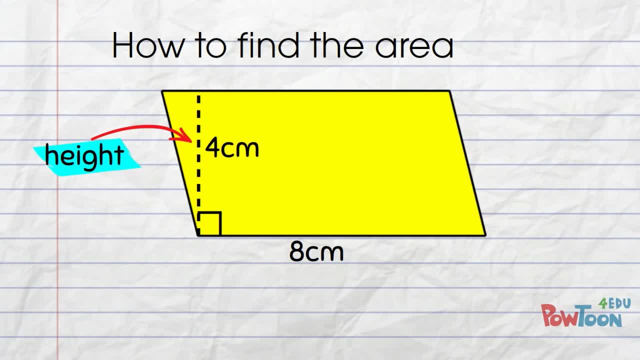 It's 4cm. Now we have measurements on two sides that meet at a right angle, So we're ready to go. The area of a parallelogram is Base times height. So 8 times 4 is 32cm squared. 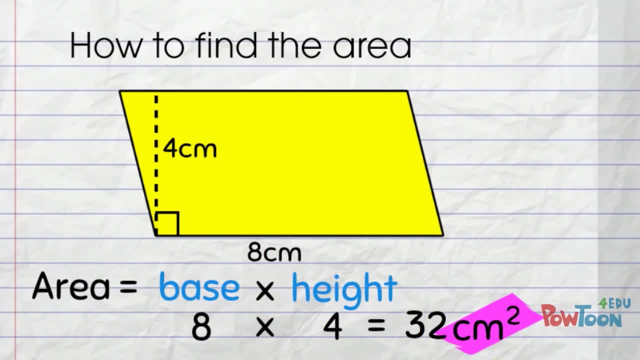 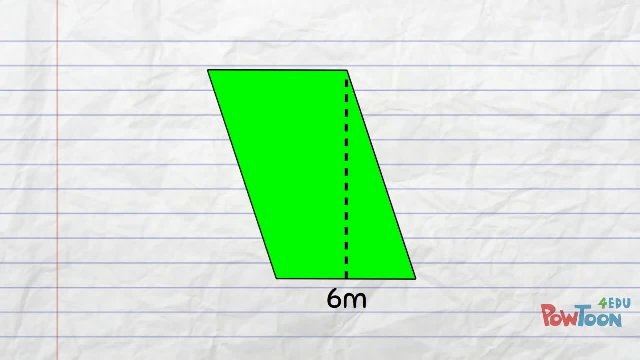 Never forget units of measurement. The height changes from D to B, So we have 7 units of measurement. I don't think it's too difficult to estimate the height of a reference. It requires a lot of study. There's also a lot of research to find out. 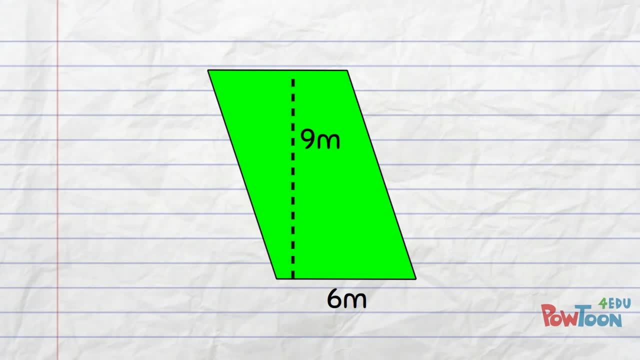 Here's the base 6 meters. Here's the height 9 metres. What about this parallelogram? Here's the base 6 metres. Here's the height 9 metres. It doesn't matter where the height line is shown.